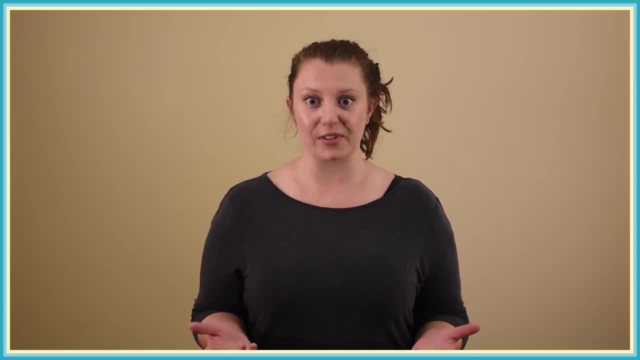 the strange phenomenon called oscillation that scientists found in neutrinos, Much like a human suddenly appearing as a honey badger. neutrino oscillations were unexpected. They're proof that our understanding of the particle world isn't finished. So today, on Even Bananas, let's talk. 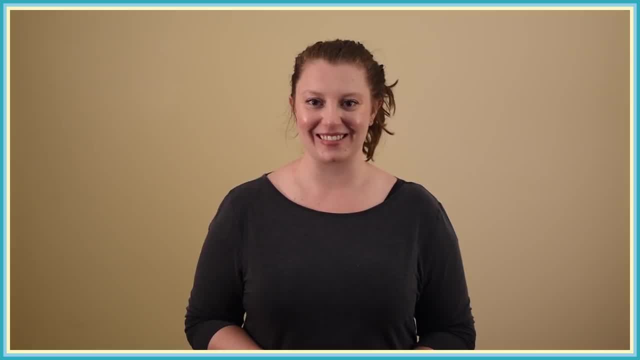 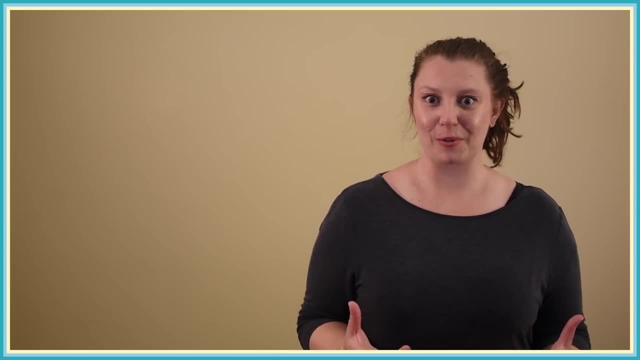 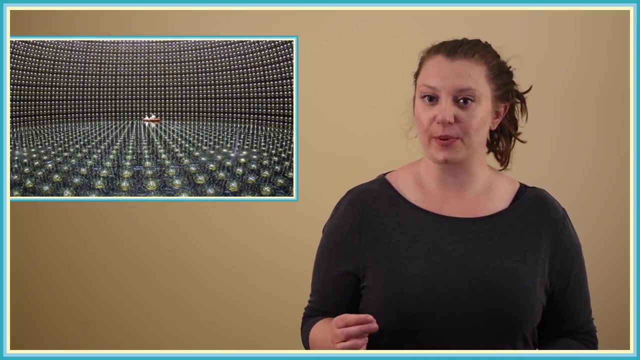 about how experiments study neutrino oscillation. As you can probably guess, neutrino oscillations are a major focus of research at neutrino experiments around the world. Some experiments study oscillation at the average speed of two year intervals and some at a higher speed. 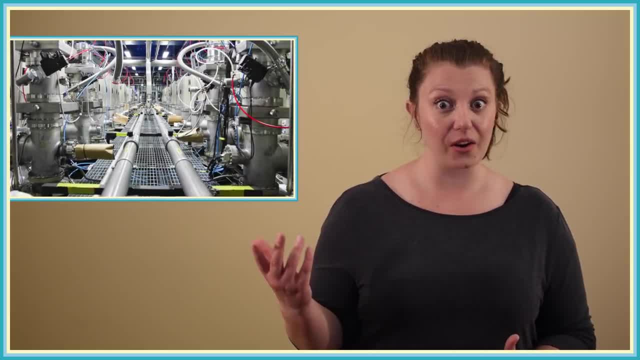 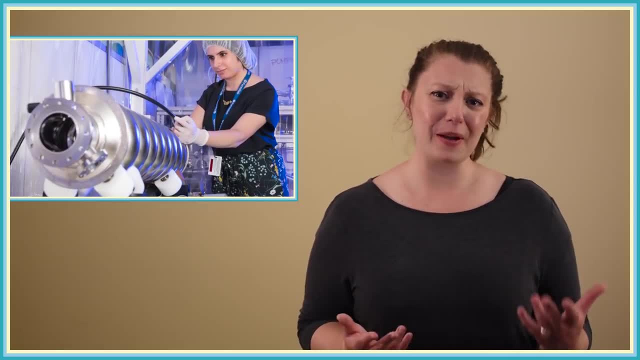 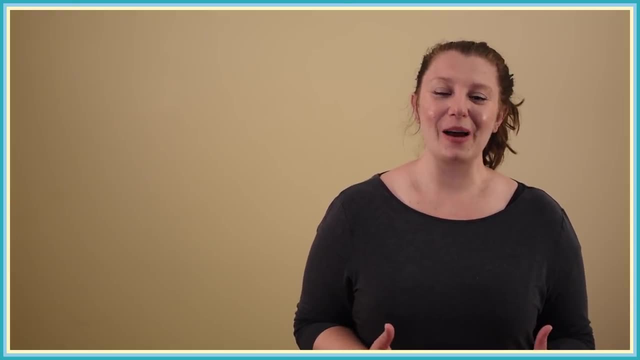 oscillating neutrinos from naturally created sources like the Sun or the Earth's atmosphere. We use particle accelerators to create a neutrino beam at Fermilab to have a bit more control over the neutrino types and an excuse to make pew-pew noises. At Fermilab we have a lot of neutrino. 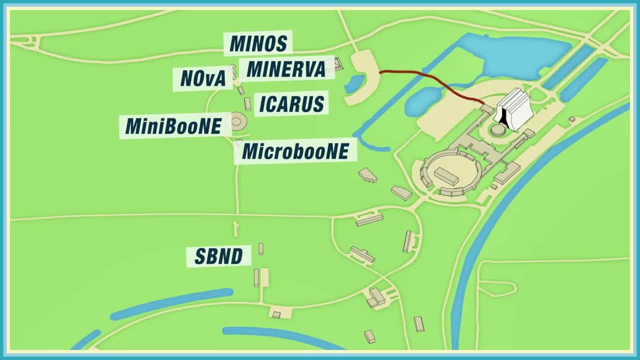 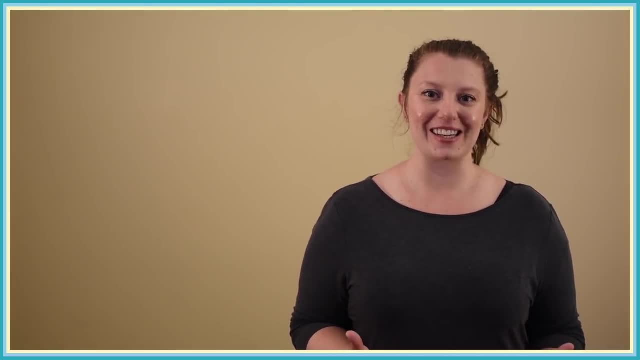 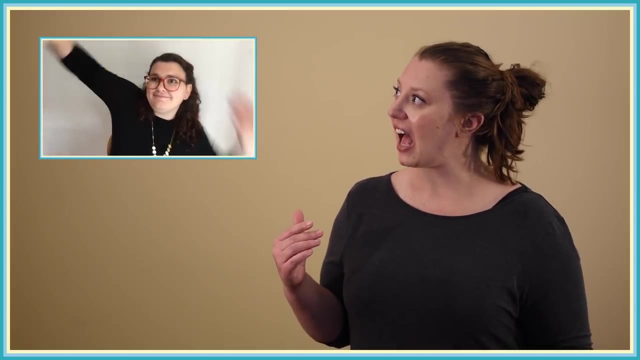 experiments that study how neutrinos behave over short and long distances To explain how our experiments study oscillations at long distances. I'm joined today by Fermilab scientist Anne Norick. Anne studies Anne, Anne, Anne, you know people are going to see this right. 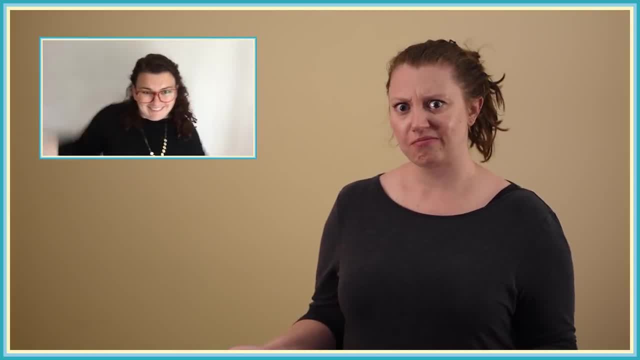 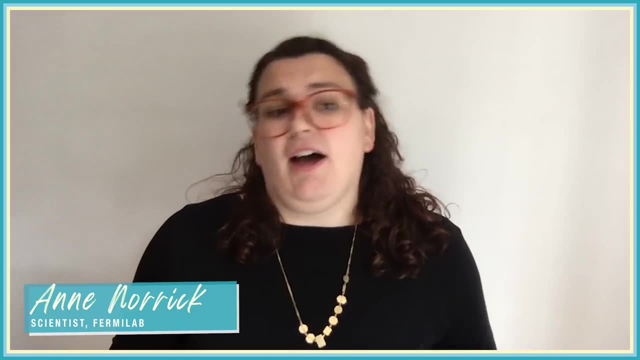 What are you doing? I'm oscillating. Hi friends, I'm Anne Norick and I also study neutrinos at Fermilab, which apparently means I'm not allowed to oscillate. I study neutrinos with the NOVA experiment and work with current experiments to study neutrinos. I'm Anne Norick and I also study neutrinos at Fermilab, which apparently means I'm not allowed to oscillate. I study neutrinos with the NOVA experiment and work with current experiments to study neutrinos. I study neutrinos with the NOVA experiment. 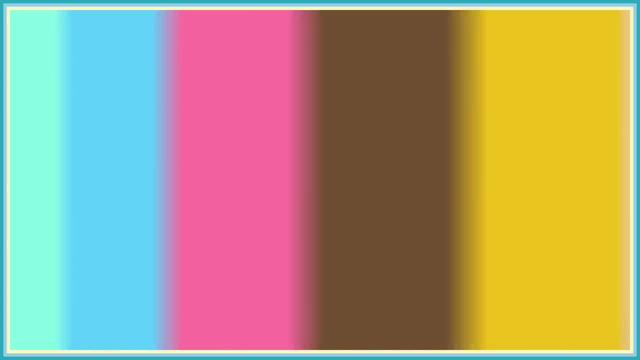 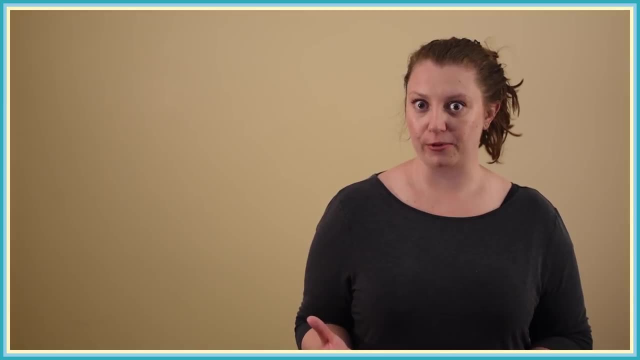 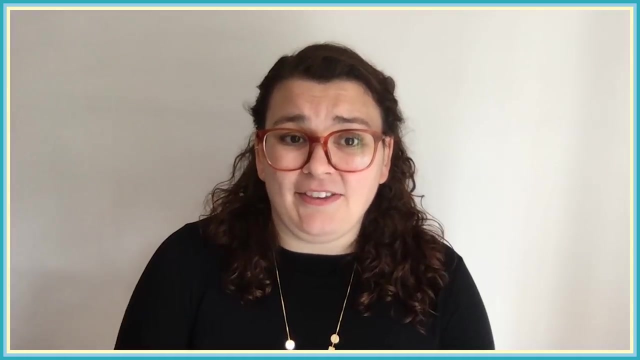 and work with current experiments to study neutrinos. When we try to measure neutrino oscillation, we're looking to see if the neutrinos change flavor as they travel. To accomplish that, some of our experiments use two neutrino detectors. This means we measure our particle accelerator neutrinos just after we make them in what we 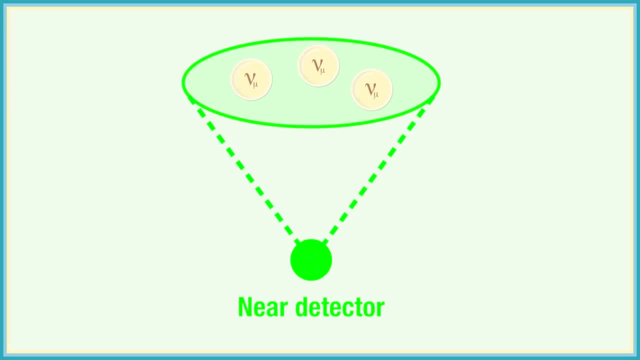 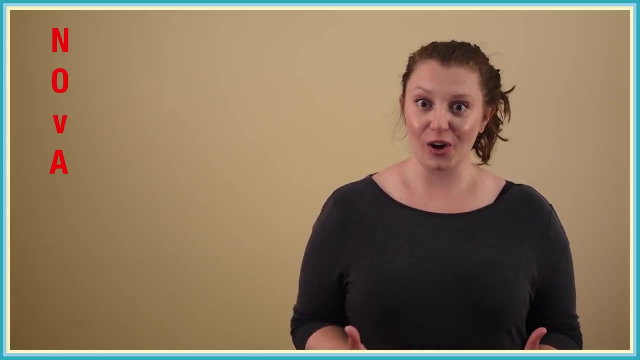 inventively call a near-detector to make sure we really know what we're starting out with, And then we measure them again at a distance to give us a more accurate and accurate measurement to see if they have changed their flavour. The NOVA experiment is making some of the world's most precise measurements of neutrino oscillation. 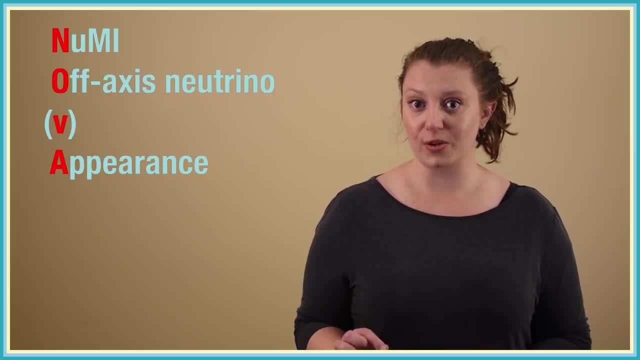 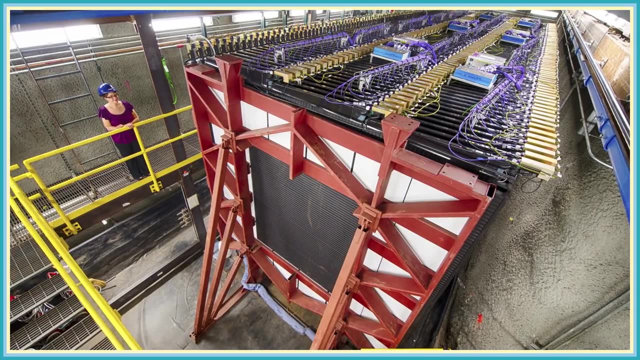 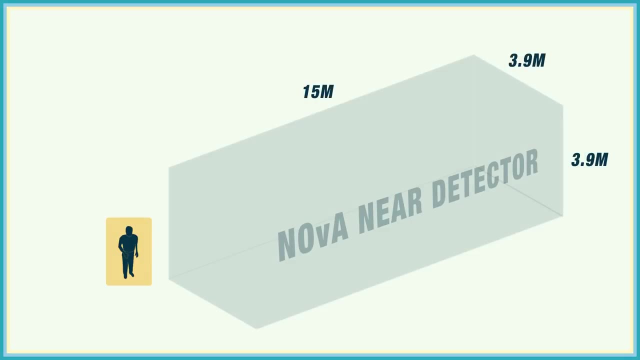 using neutrinos from Fermilab's NUMI beam and a two-detector system. Roughly one kilometre away on the Fermilab site sits the NEAR detector, 100 metres underground. It's made of 300 metric tonnes of plastic, mineral oil and scintillator. 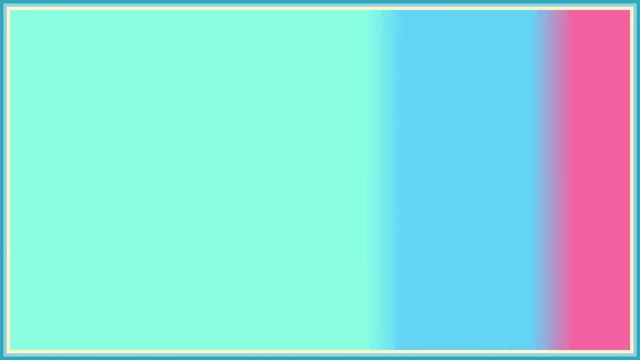 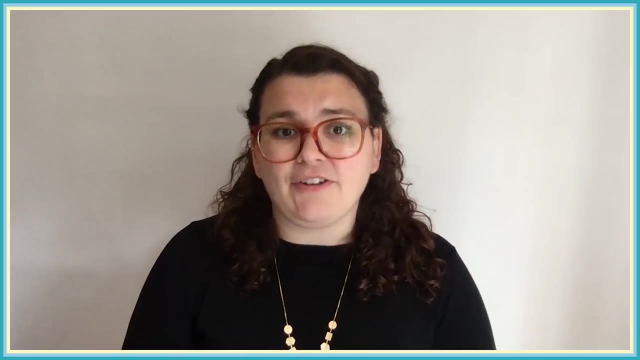 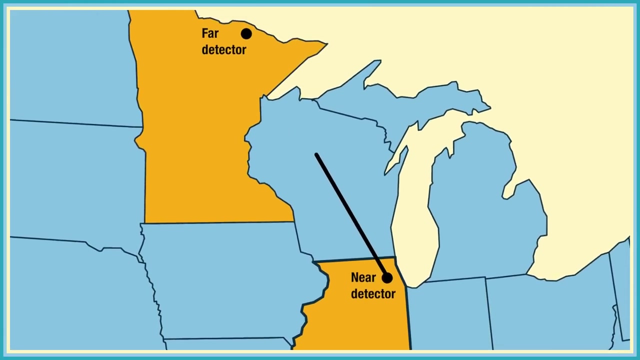 Sections of it light up as particles interact in the detector. The neutrino beam is very dense at the NEAR detector so we see a lot of particle interactions. We collect data on their energy and flavour. The neutrinos that don't stop in our NEAR detector continue on about 500 miles up to the FAR detector in Ash River Minnesota. 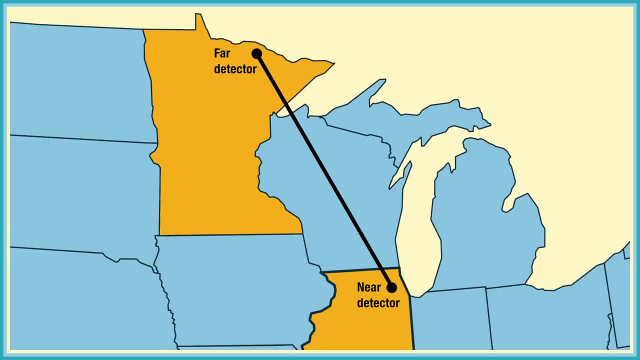 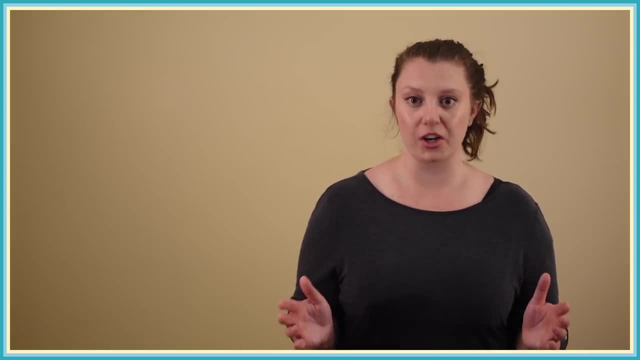 The whole trip takes them less than three milliseconds. Similar to a flashlight, the neutrino beam spreads out as it travels, so the FAR detector needs to be much bigger. NOVA's FAR detector uses the same materials but weighs 14 metric kilotons. 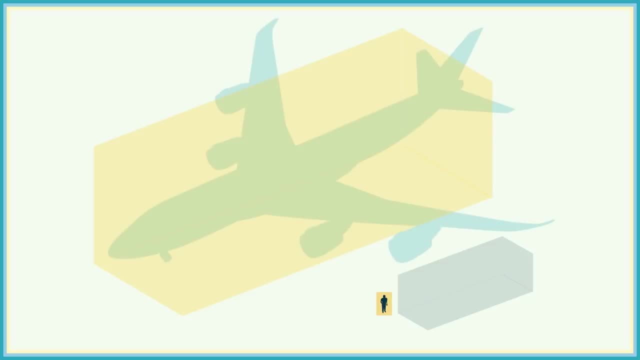 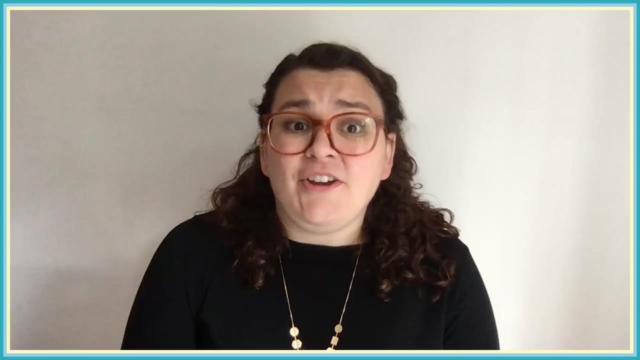 and is about the length of a commercial jet. Making both detectors out of the same materials makes it easier for us to compare the neutrino interactions we see. When the neutrinos get to Minnesota we check to see how many of them have oscillated. 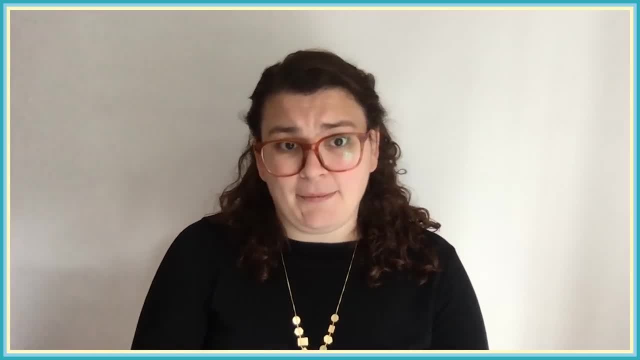 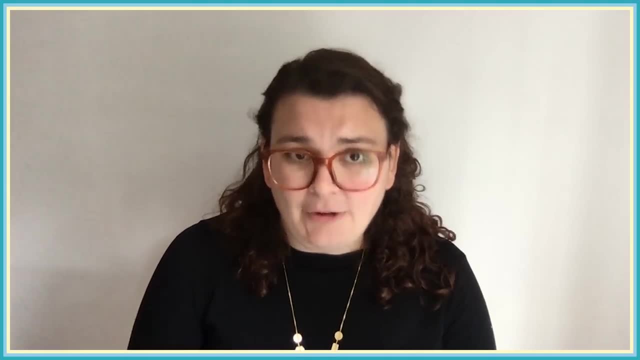 At the NEAR detector, 99% of the neutrinos in our beam interact as muon neutrinos, but by the time they arrive in our FAR detector, almost all of them appear as electrons Or tau neutrinos, And that's not a coincidence. 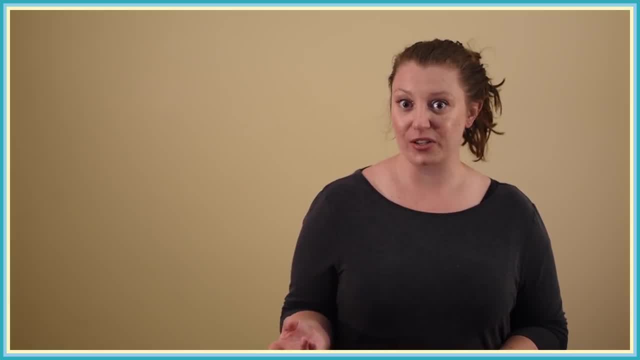 We build our FAR detectors where we expect, lots of neutrinos will have changed their flavour In our marathon analogy. if you wanted to see a human change into a honey badger- and who doesn't- you'd stand wherever the math says is optimal honey badger zone. 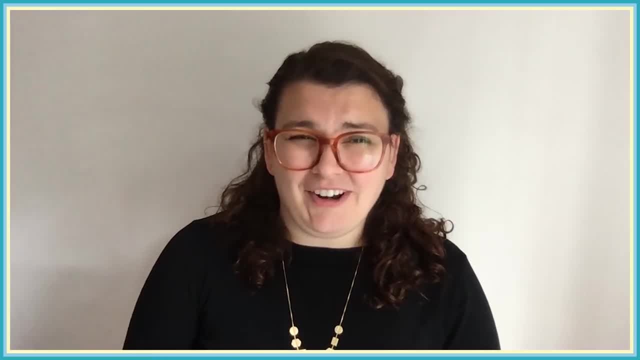 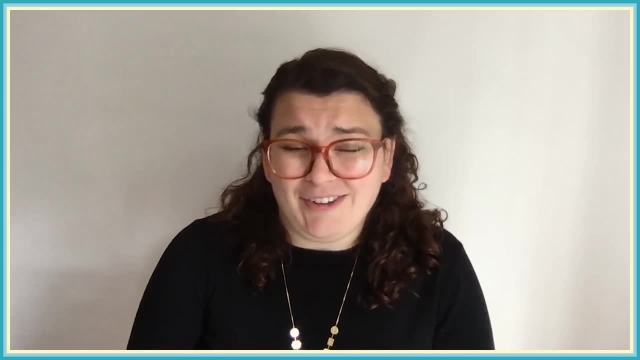 It's very difficult for us to find tau neutrinos in our detector because tau leptons are really heavy. Most of the neutrinos in our beam don't have an effect on us. They don't have energy to make a tau lepton. 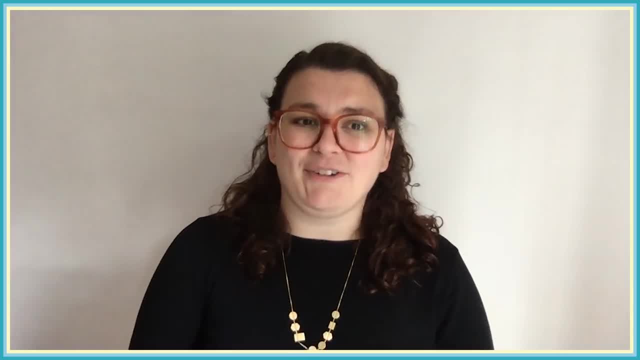 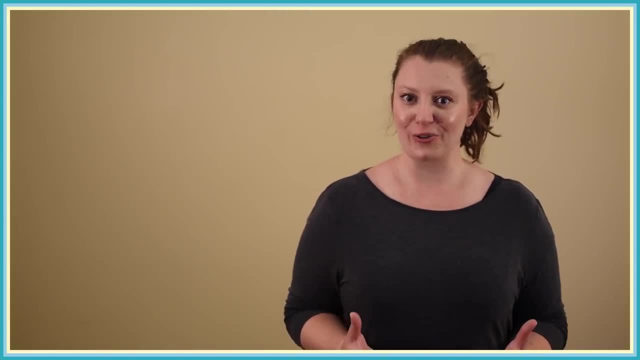 So to us they're pretty much invisible. But NOVA can see electrons created by electron neutrinos that have appeared in the beam through oscillation. So that's what we look for. One of NOVA's main goals is to see if neutrinos oscillate differently from anti-neutrinos. by comparing measurements from a neutrino beam and an anti-neutrino beam. So far, there are some hints that they might be different, but we need a lot more data before we can be sure. In the future, we're planning to get loads more information about neutrino oscillation.